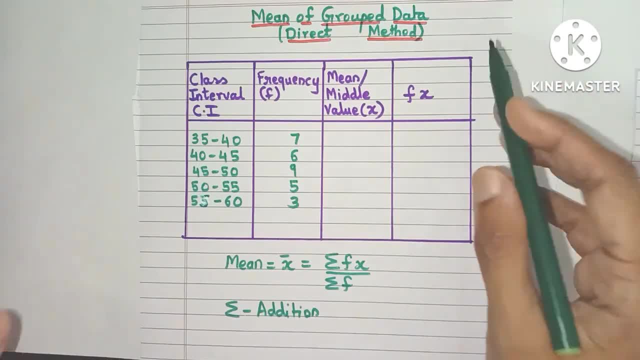 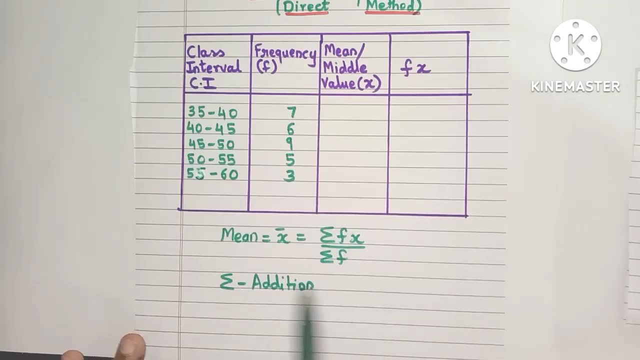 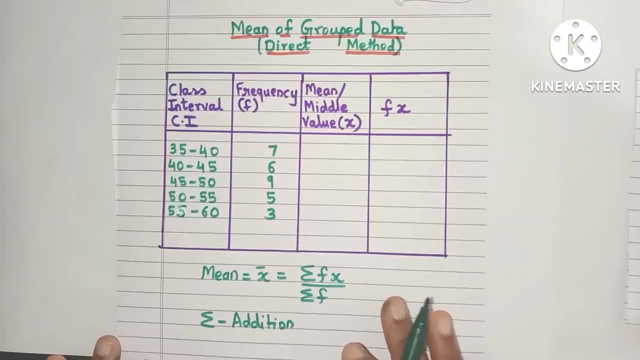 Hello everyone. Today let's learn how to find the mean of group data. So, friends, in this example, here is the class interval column and this is the frequency column. Now the formula is mean or x bar is sigma fx divided by sigma f. Now, friends, before we can use this formula, we need two more. 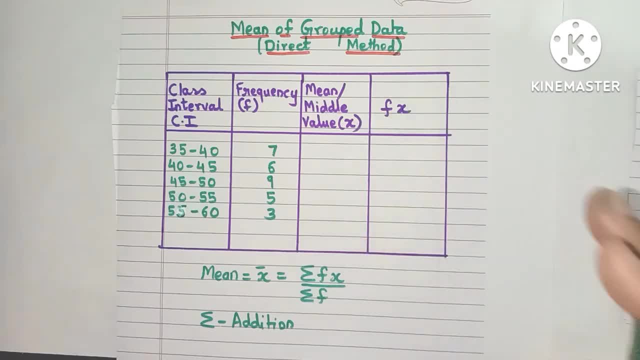 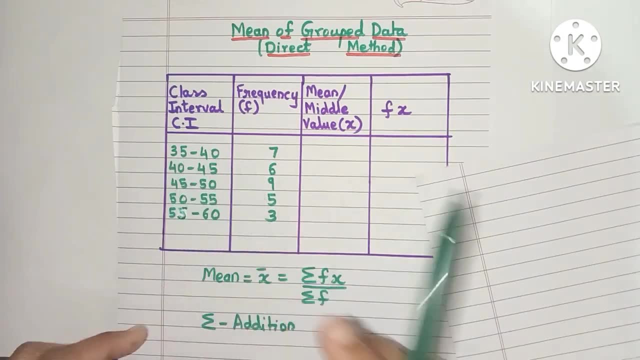 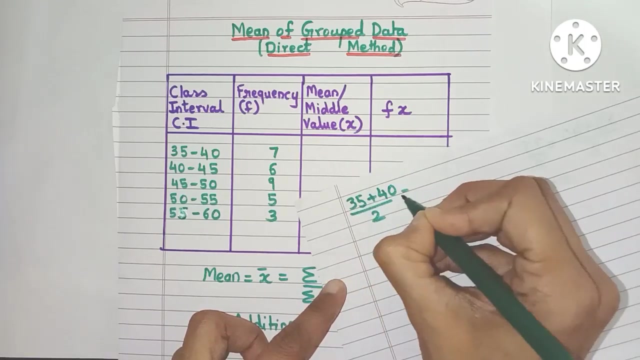 columns. So the first column is the x column. Now, what is x? x is nothing but the mean or the middle value. So we find x by adding the upper limit and the lower limit and dividing it by 2. So for the first class interval we have 35 plus 40 and divided by 2 friends. So 35 plus 40 is 75. 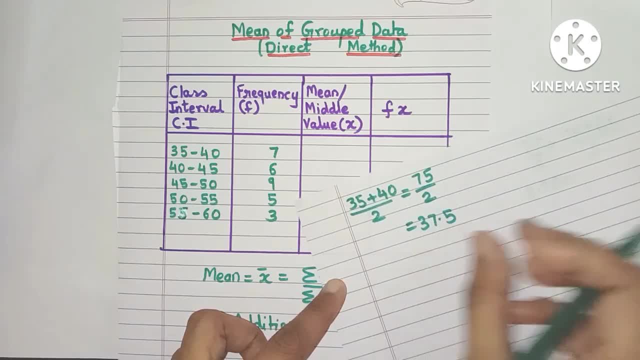 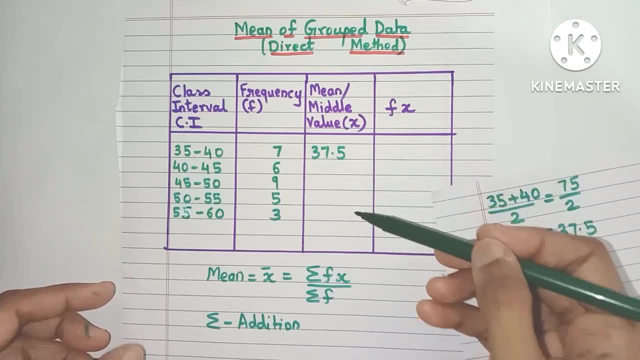 divided by 2, which will give you the answer is 37.5, and this is your x value for the first class interval. So, friends, this way you can find the x value for all the class intervals. but usually an easier method is used. So, after finding the x value, 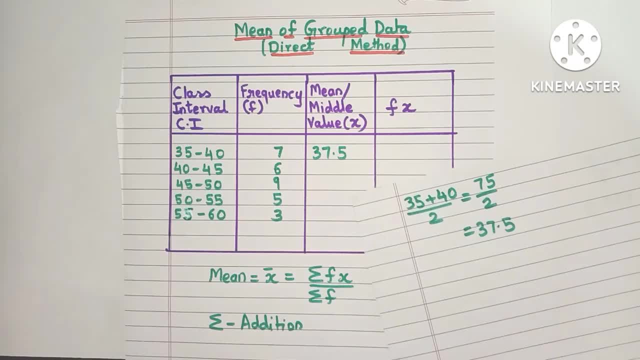 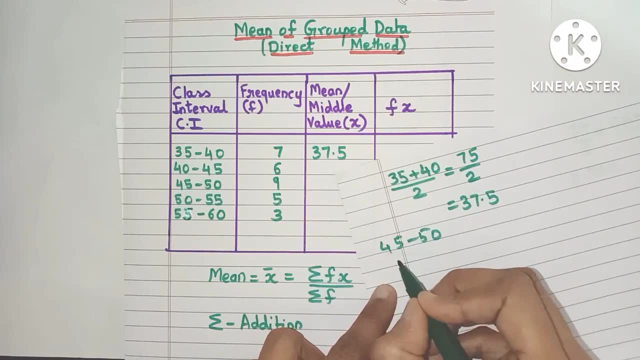 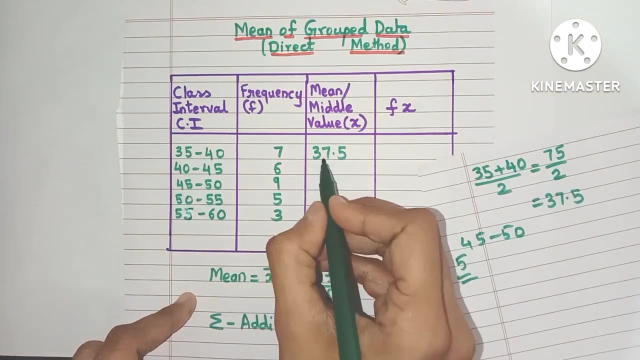 for the first class interval. in this way: just find out the class size. So any class interval, say suppose 45 to 50. What will be the class size Upper limit minus the lower limit, which is 50 minus 45? that is 5.. Just add this 5 to this x value, friends. So 37.5 plus 5 you will get 42.5. 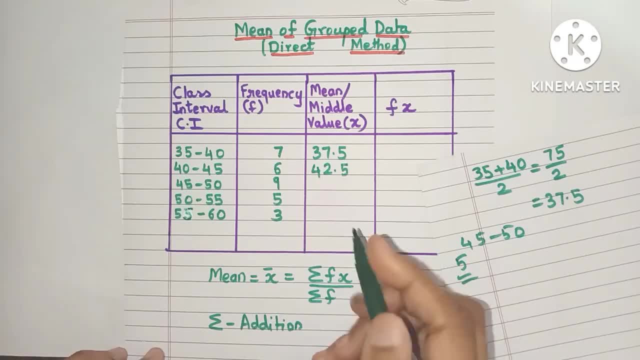 and this will be your next x value. So it's a very easy method. Similarly, just add 42.5 to 5, you will get 47.5.. So this way you can find the x value for the first class interval in this way. 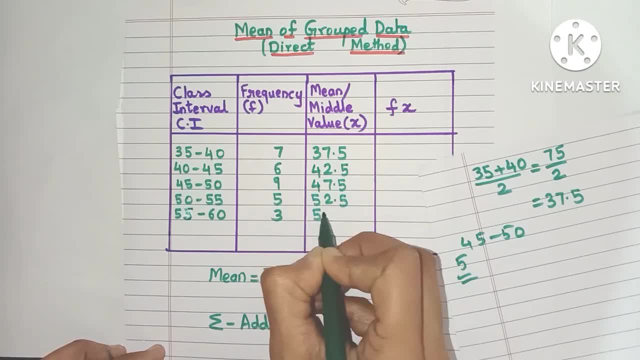 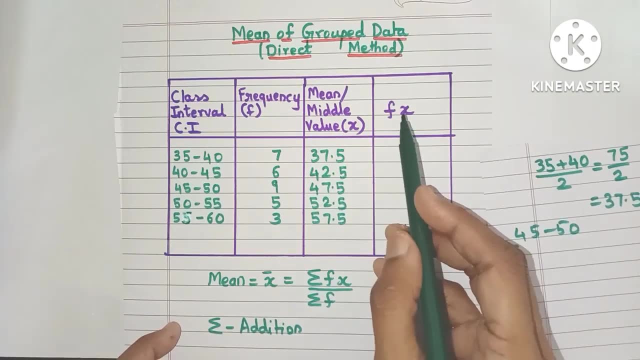 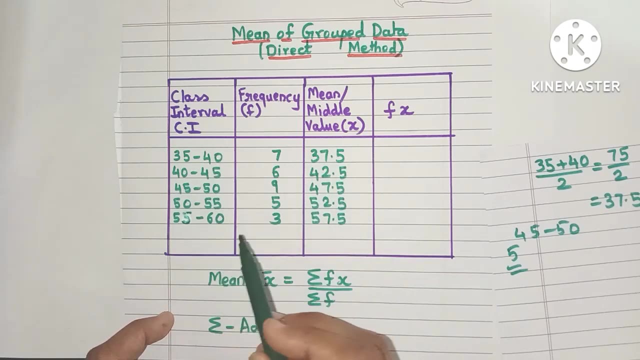 7.5, then you will get 52.5 and 57.5. so this way you will get the x values for all the class intervals. now we need to add one more column called the fx column. so in this column we simply multiply the f value and the x value for all the class interval. so, friends, for the first class. 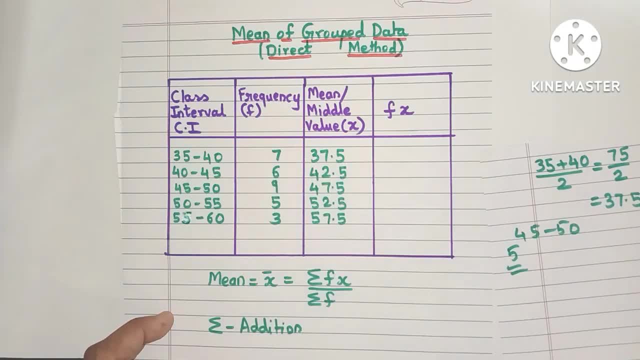 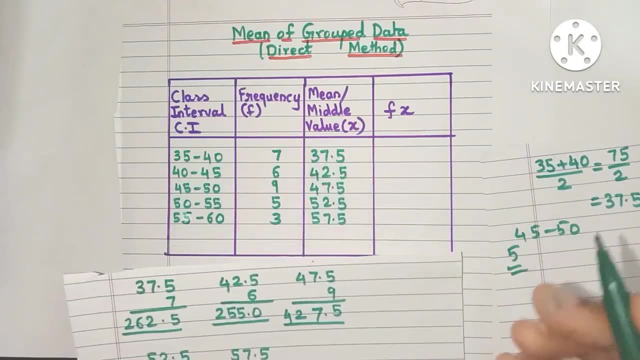 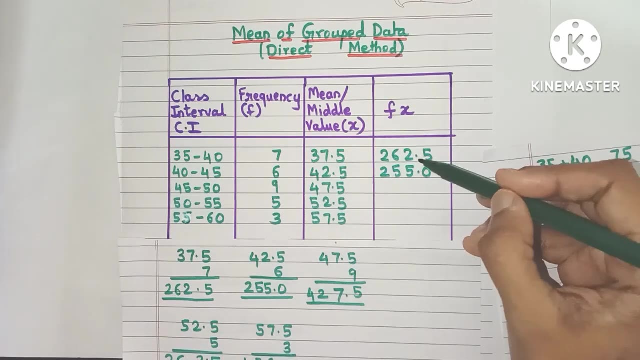 interval. i will simply multiply 7 and 37.5, so save time. i have already done all the calculations where i have multiplied the f value and the x value, so let's quickly note it down. so here i have 262.5, then i have 255.0. and friends, one thing to be noted is that you need to place the decimal.